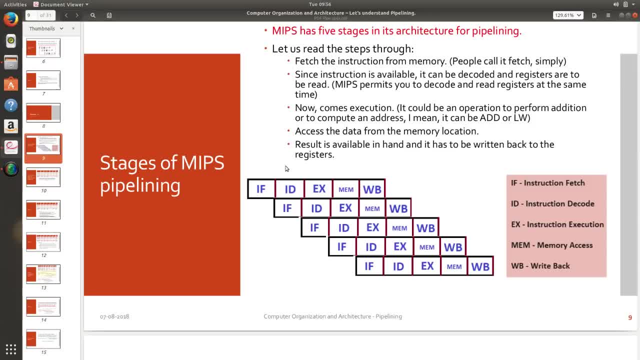 And MIPs has got a special ability to decode and read the registers at the same time, So we do not have a separate stage To read the, instead read the contents from the register. for example, if it is R type instruction, we may have to read the content from the register. 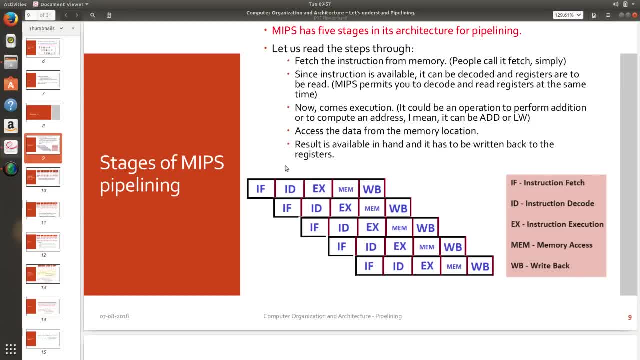 R, S and R D, RT, etcetera. So that can happen easily through this stage itself, where the instruction is decoded as well. at the same time it is the register content is also read. The next stage is called as execution, where based on what instruction are you using? 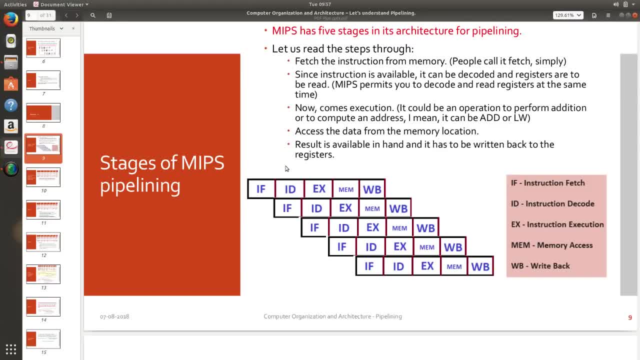 For example, if it is an ADD instruction, the source register should be added and then the result should be available for you. that process of alu being involved, that process of computing, the result happens in the third stage, the fourth stage, if you are going to a memory. 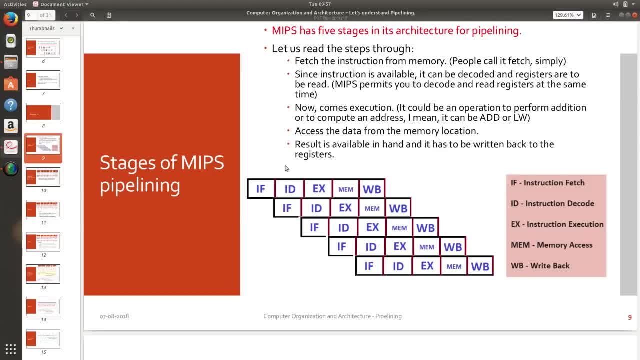 location, for example a store and store word instruction or a load word instruction, we may have to go into memory location to fetch data or to store the content there. so in that case we will have to access memory and that is called mem, which is the fourth stage. the fifth stage is referred as: 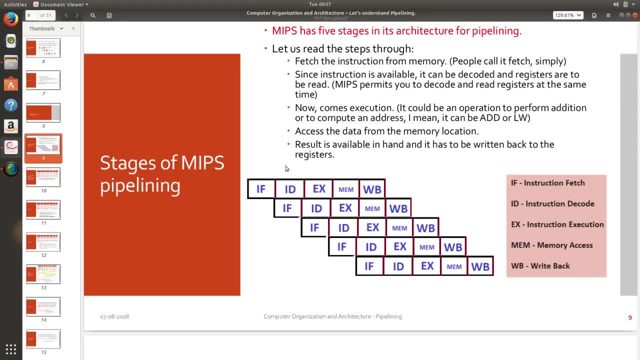 write back. you need to write the result back into the destination register. for some operations like uh add, add immediate, etc. you are going to write the result back into the registers which are assigned as the destination register. so now five stages are there: instruction, fetch, instruction, decode, execution stage, memory stage and write back. now, if it is pipelining, how? 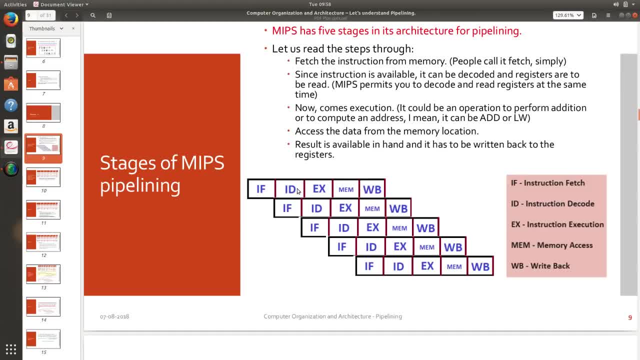 it will look like you can see that here. first stage is instruction fetch, second is id, third is ex, fourth is mem, fifth is write back. when the instruction fetch is done, the second instruction will start instruction fetch and the first instruction will go to id. when the first instructions exe stage is happening, the second instruction can start with the id. 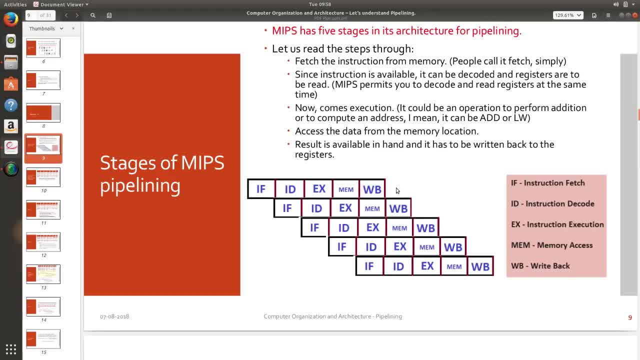 whereas the third instruction will start with. if, likewise, it will keep going on and you can see that there is a layer like structure here, and by the time we complete the first instruction, the fifth instruction should have started this first stage. so that's the point here. so we have got five stages here. so by the time the first instruction is getting into the last stage, 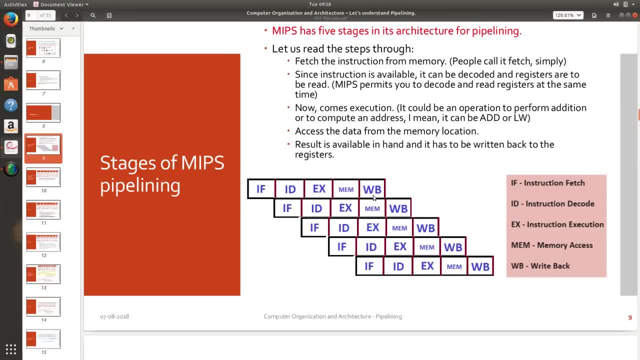 the fifth instruction will get into the first stage. this is called pipelining, and assume that each instruction takes about ten minutes to complete independently. when they are executed one after another it will need fifty minutes, but here it could be much lesser. so that is the crux of pipelining and i hope you understood. 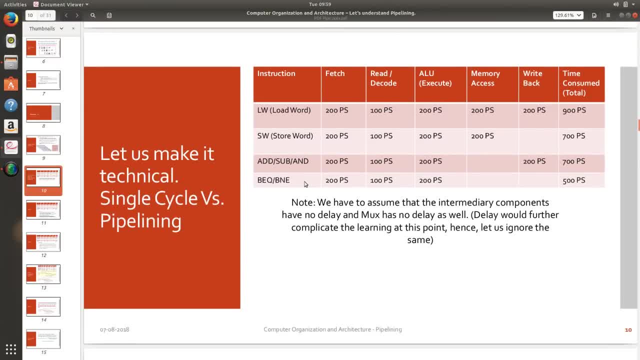 the stages of pipelining. let us take a very simple example here. let us let us make it more mechanic, more technical, whereas we can compare how exactly it works with a single cycle and how exactly it goes on when you have a pipelined architecture. it is a very 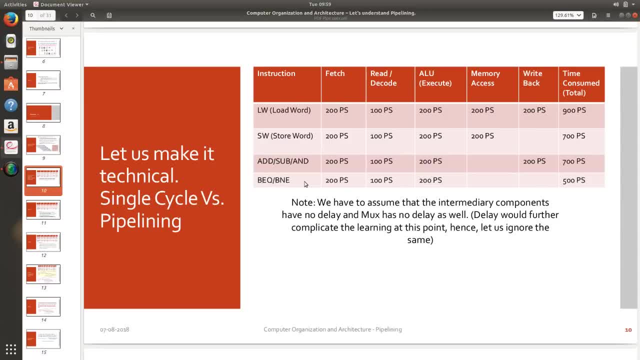 simple example what we have given. we have taken load word and it takes two hundred picoseconds for fetch, hundred picoseconds for read, two hundred picoseconds for ALU, two hundred picoseconds for memory access and write back. it needs two hundred, so totally nine hundred seconds. 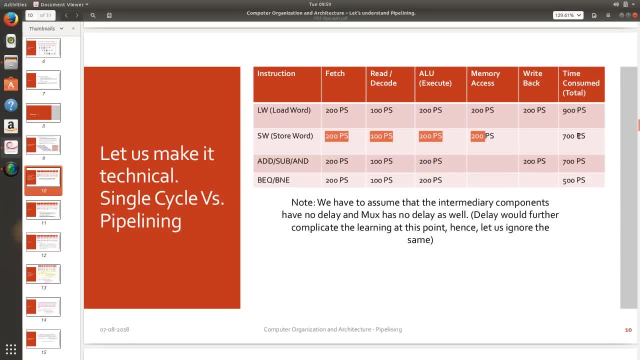 is needed for load word. similarly, store word needs seven hundred picoseconds, add, sub and all those kind of operations need seven hundred and BEQ BNE need five hundred picoseconds. this data is random and this is just for enunciation and this is just for understanding and most important point that you need to look into. 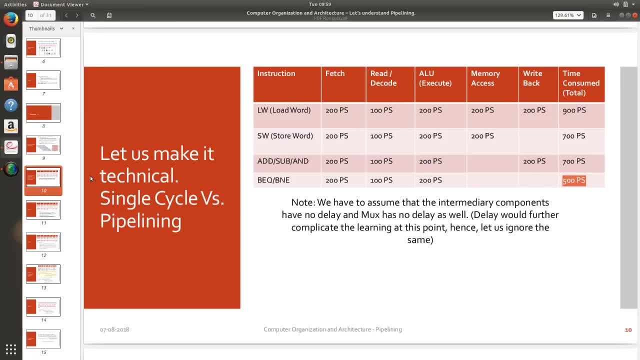 here is: we have not considered that any delay would be incurred in between the stages or the multiplexers would cause some delay is not been considered. so it is considered that all the output or all the stages that are given with some time here are all ideal, which 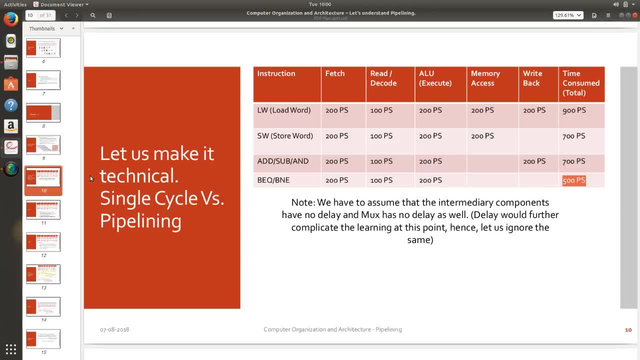 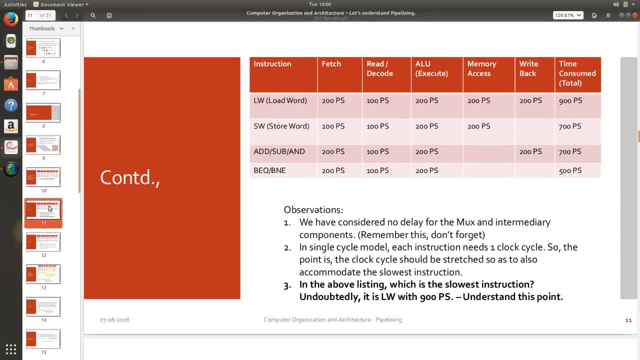 means it has got no delay. so this has to be understood very clearly. if this point is forgotten it would be probably a trouble. so we are considering hundred percent ideal condition. so we are considering hundred percent ideal condition. now what will happen? very simple: we have considered no delay. as i told you, in single cycle model, we know that each instruction will need one. 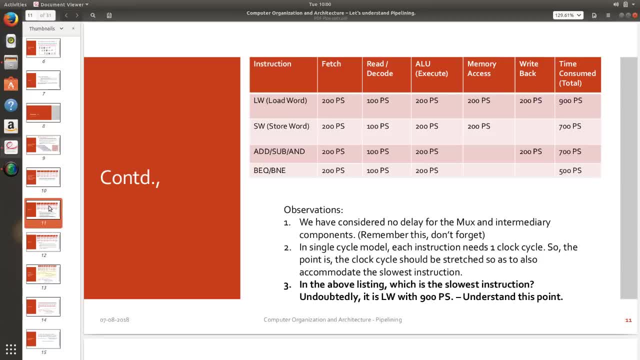 clock cycle. this is the base of single cycle model. each instruction would need one clock cycle, so the clock cycle should be stretched so as to accommodate the slowest instruction. what do you mean by that here? the fastest instruction needs only five hundred picoseconds. medium instruction takes about seven hundred picoseconds. these two and the slowest instruction. 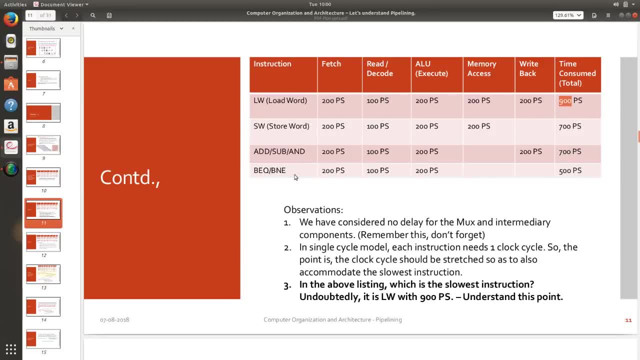 is nine hundred picoseconds. what is the slowest instruction? it is the slowest instruction. it is the slowest instruction in the one of the slowest instruction in the result here. in the instruction set here, it is nothing but load word. so it is to be understood very clearly. 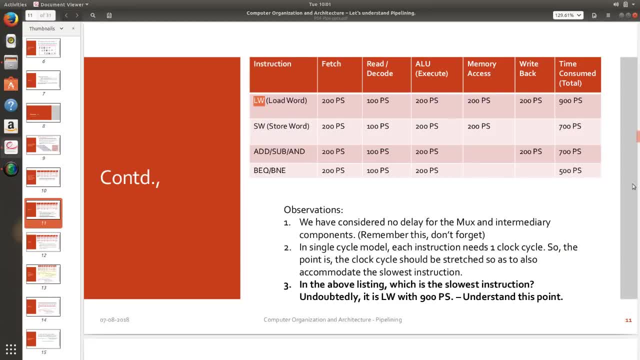 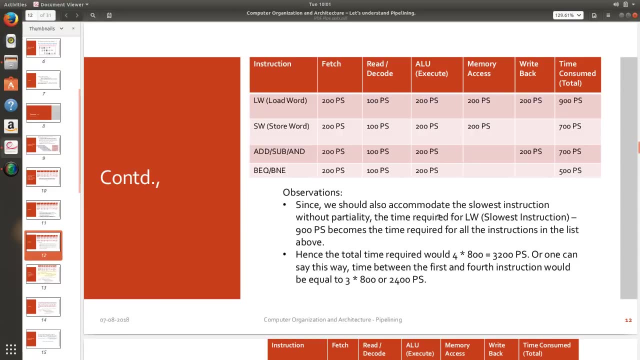 that single cycle model cannot work with just taking this lowest of the data. it should also accommodate this longest of the time that is needed by the instructions to survive. so what is the impact, sir? the impact is very simple, since we should also accommodate the slowest instruction. now nine hundred picoseconds will become the time for all the instructions. 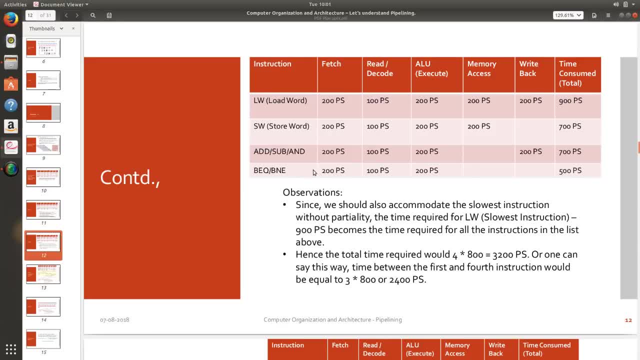 in the list here. what i mean to say is, though it is five hundred picoseconds, it will not be five hundred picoseconds. instead, it will be nine hundred picoseconds, because it has to accommodate this as well. this is a very, very important point. now, what will happen? 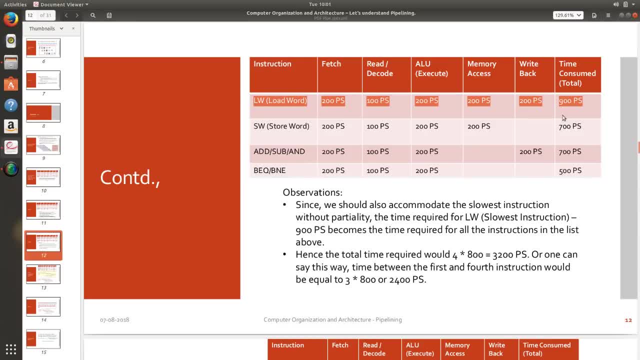 for us to compute all these four instructions, it would need four into nine hundred, which means i have made it a mistake here. four into nine hundred, which means it is three thousand six hundred. or we need to three into eight nine hundred, which means two thousand seven hundred, to reach the final stage. this is a very important point. please 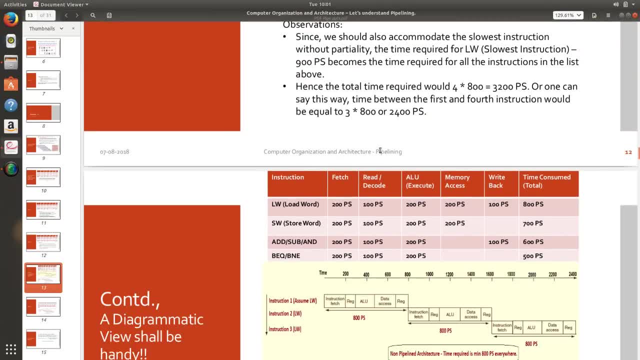 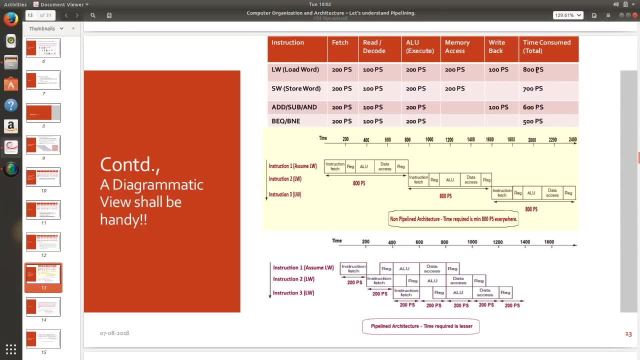 remember and do not forget whenever we talk about single cycle, it will become a problem. now let us go into the pipeline architecture. here you can see that a load word has got, say, about eight hundred, store word has got about, say, somewhere close to seven hundred. add sub etcetera has got six hundred. beq has got five hundred. the same data that i am taking. 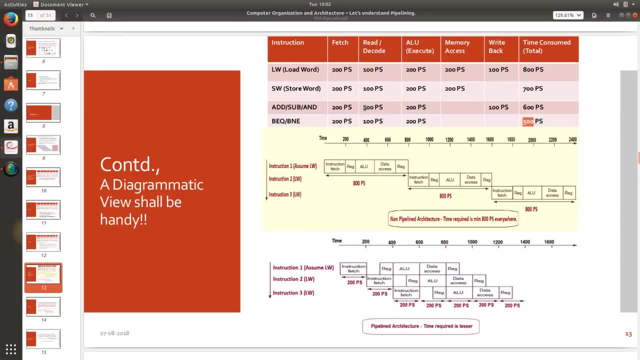 maybe some slight variations could be there. forget about the slight variations, not a problem. now understand that when we go for pipelined architecture, non pipelined architecture will require this way will be executed. wait. second instruction will be executed. gone third instruction will be executed. so 800 plus 800 plus 800, 800 being the maximum of the time. we need to accommodate that time as the 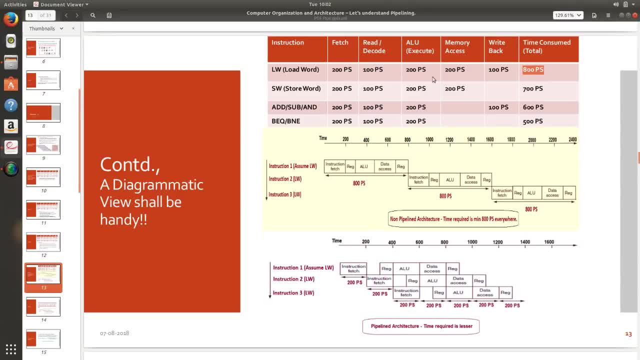 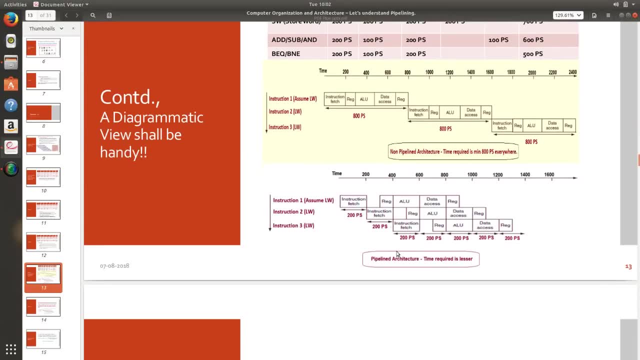 time required for any instruction. this is what i told you in my previous slide. it can be 800 or 900, whatever be it, whatever is the biggest count there, you need to take it up as the reference and it will work that way. now let's go to the pipeline architecture. you can see that here. so what will? 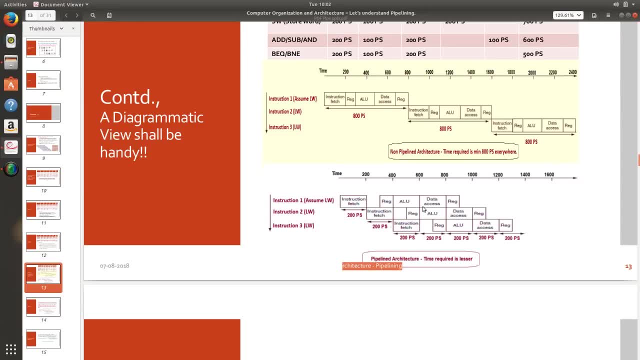 happen is very simple. the time liquid is lesser, so i can complete the first instruction and when the first instruction fetch- is over, my second instruction will start. then the third instruction will start. the ladder like structure, the footstep like structure has come, but there is one small. 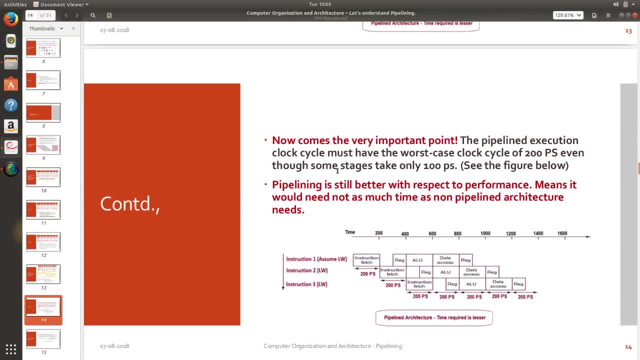 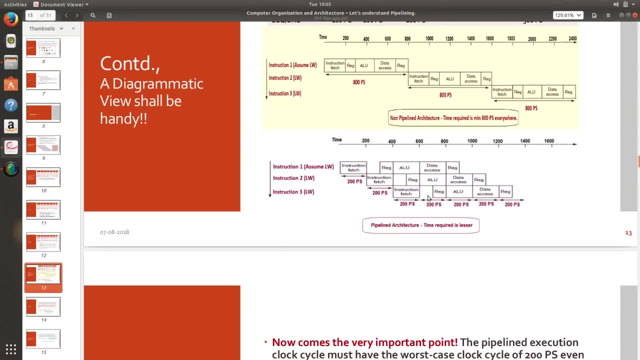 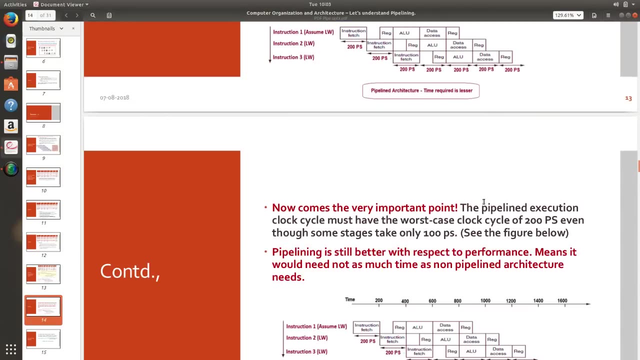 catch. here. now comes the very, very important point: the pipeline execution clock must have the worst case clock cycle of 200 picoseconds, though some stages take only 100. for example, this stage needs only 100, but i will take the worst case as 200, since the rest of the stages need 200. so what? 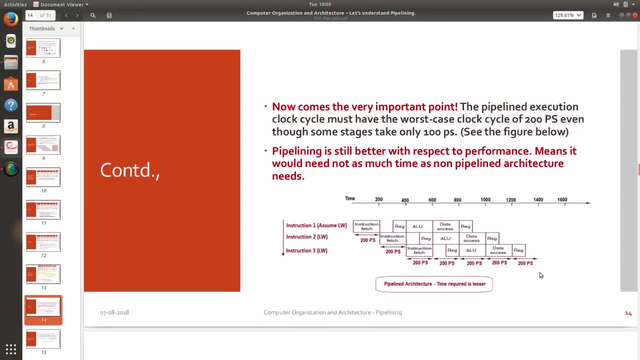 will happen is every stage will be given 200, 200, 200, 200, though they need only 100, but overall, if you see, it is still a better performance there. you have seen, you have taken the worst case of 800 picoseconds for one instruction and you had to. 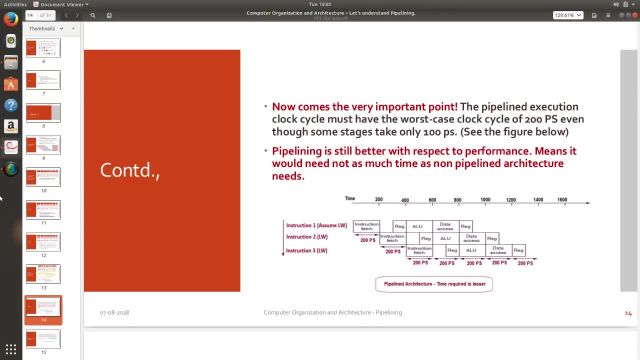 accommodate rest of the instructions, even with the same size. but here what we are talking about is the stages. what we are talking about is the steps, and if one stage needs 100, it will not be considered. if another rest of the stages need 200, 200 should be considered. so it should be 200 for each of this. 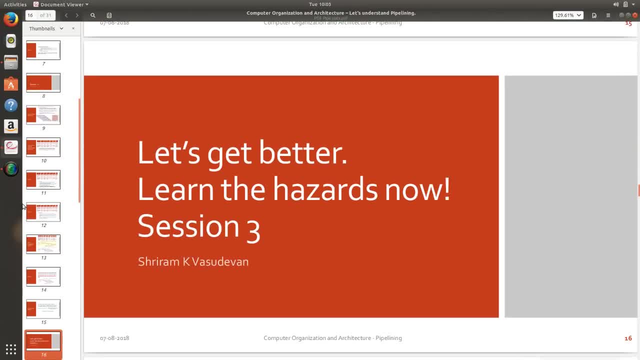 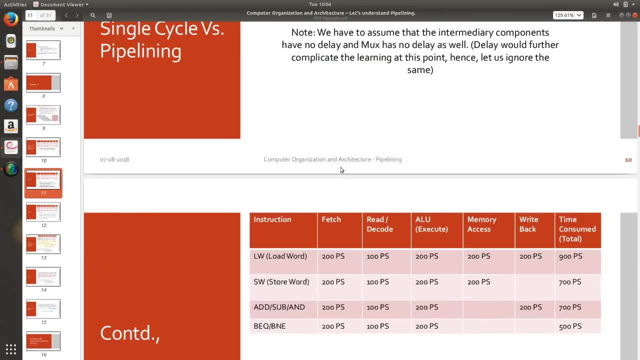 stages. in either case, it will be much more better than the previous attempt. so let's get into the next session, where we will talk about the hazards shortly. what i explained in the session is very simple. i'll quickly give you a recollect of whatever we have taught. we have got five stages. 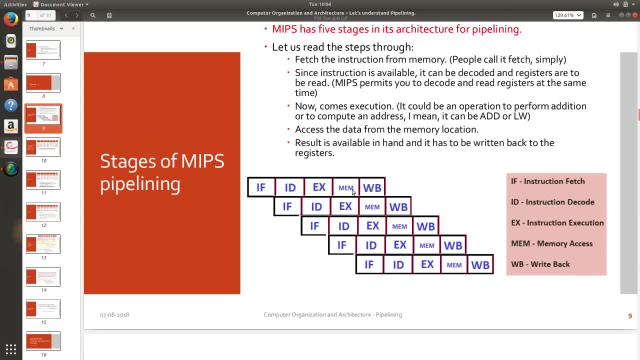 each stage being named as instruction, fetch, decode, execute, mem and write back. all these stages are called as stages. please remember the term. they are called stages and if the first stage is over the second instructions, first stage can be started, and this is called pipelining, and then 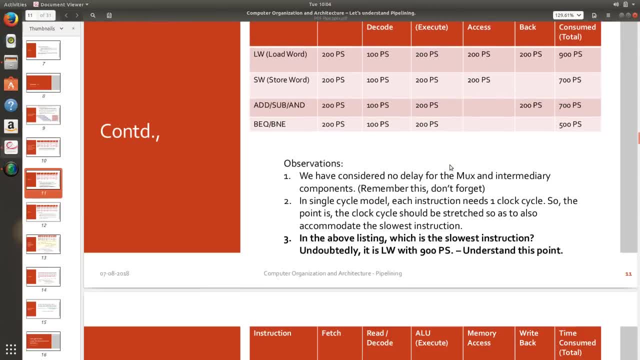 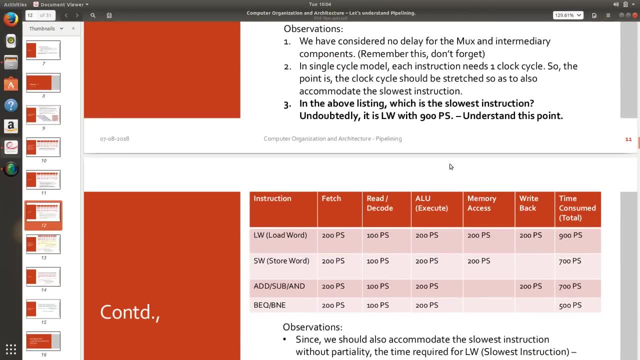 we did is we took a simple example and we explained how exactly things go for a single cycle architecture and pipelined architecture. it's a very important point to remember. do not forget: single cycle architecture will take the biggest of the time frame, for example, if it is 900 for the 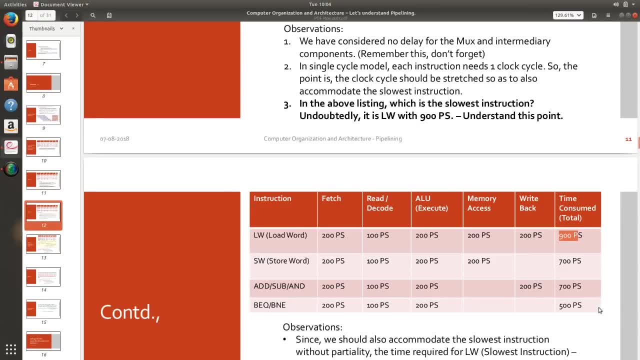 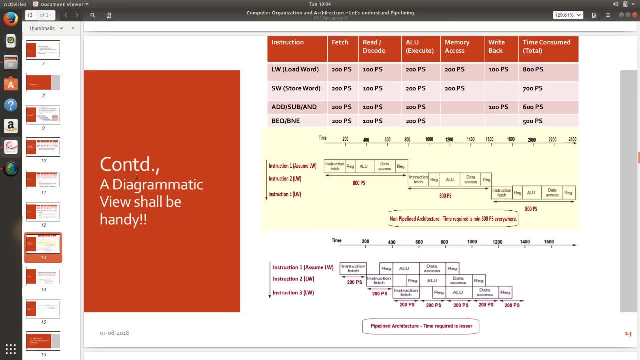 one instruction. it will take that worst case and then it will accommodate rest of the instructions also with the same amount of time. but pipelining is not so it will take only the stages and then it will accommodate. let's get into the next session where we will see more about the 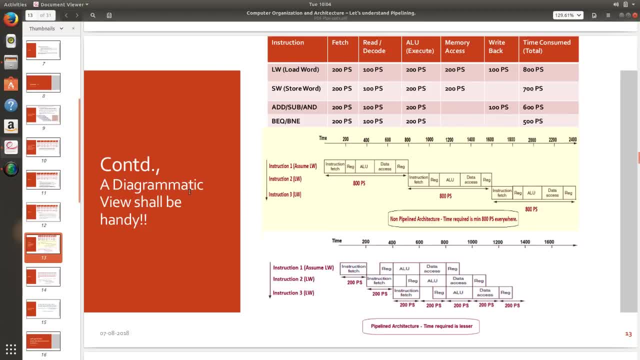 pipelining hazards. thank you very much for following my channel. if at all you have any query, you can let me know or you can put a comment. you can use your comment option and update your comment there. if you like the channel, please subscribe. thank you.